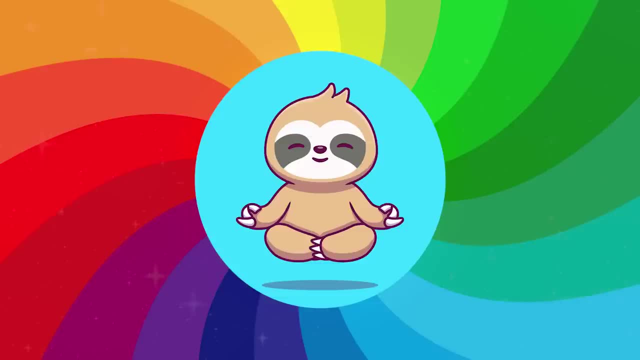 power of your mind. imagine that wherever you shine the mindful rainbow, that's where your attention goes to you. now direct the end of the rainbow and trees. now direct the end of the rainbow and trees so it shines down on your breathing. as you focus on your breathing, notice your 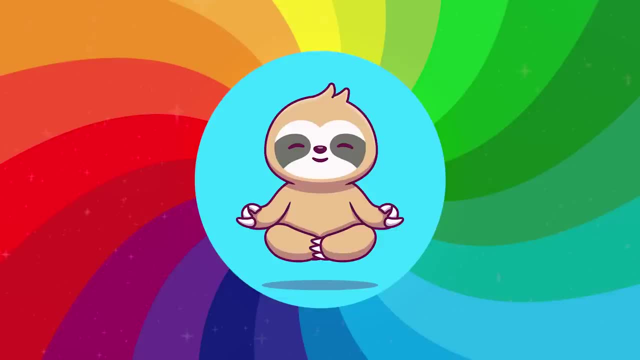 breath as it flows in and out so easily. just feel your body breathing in and out. now shine the mindful rainbow down to your feet. well done. feel your feet as they are resting on the ground. can you feel the energy in your toes? when you are ready, glow the magic rainbow on your whole body. 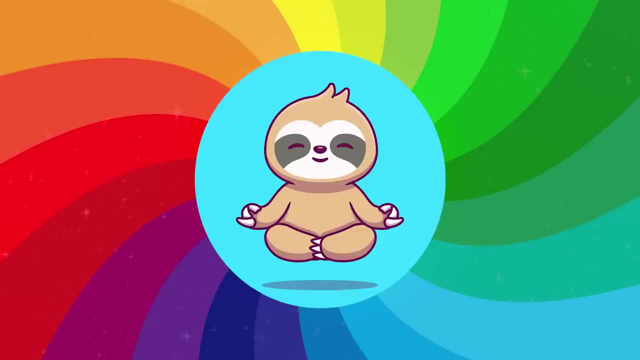 rainbow beams are shining down over your face, over your shoulders, over your back and over your belly with so many amazing colors. feel your life energy in the wonderful light of the rainbow. now, when you are ready, shine the magic rainbow inside to your feelings. take a good look around and see. 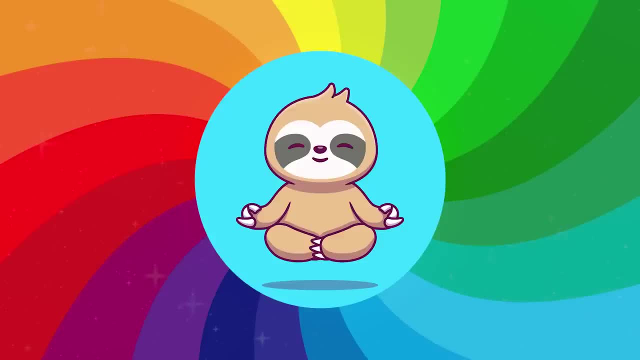 inside to what is there. so your feelings might have a color, a special color of the rainbow. so as you glow the rainbow on your feelings, what do you see? how much space do they take up? all of your feelings are welcome here. just notice your feelings as your.